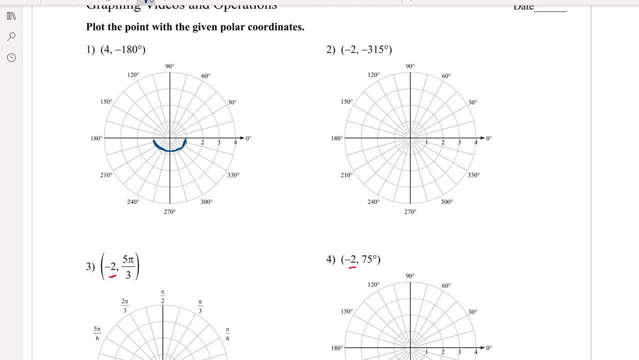 going to start here at zero and we're going to go in the negative direction. So negative 180 is the same as positive 180, but we went in the negative direction, right. And then we go out: radius of 4.. All right, so one, two, three, four. So this right, there is 4 negative 180. 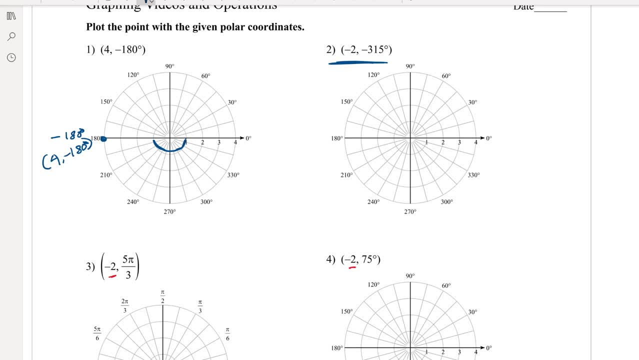 But what happens here when you have a negative radius? All right, so we're going to find negative 315.. Positive 315 is a 45 degree angle If we in the fourth quarter. so if we go negative, we're going to go. 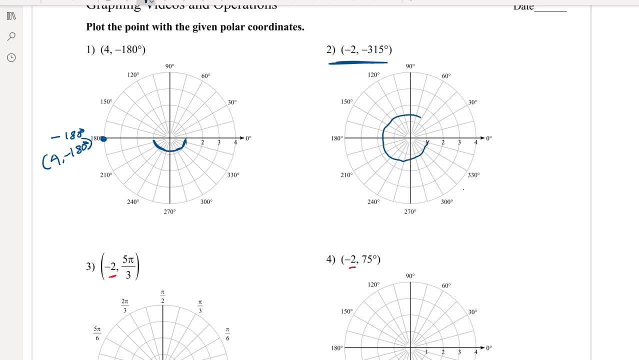 in the negative direction, to the fourth quarter, to the 45 degree. So this 45 degree angle is also negative 315.. You could also do that by. anyway, that's okay, But it's this angle, but we have a negative 2 radius. So instead of being 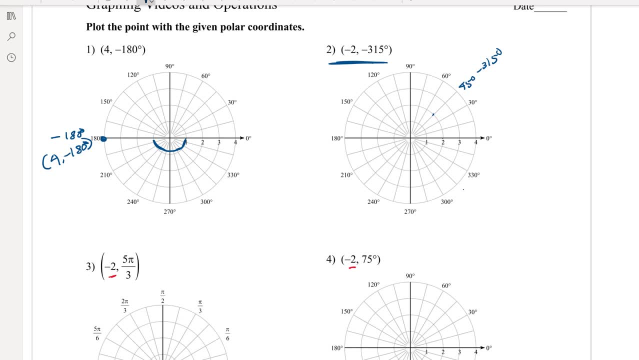 here. you now go in the negative direction. So we're going to. so imagine you had this angle and you carried it all the way through and you go to negative 2 and then follow it down to that angle. That's that point, right there. 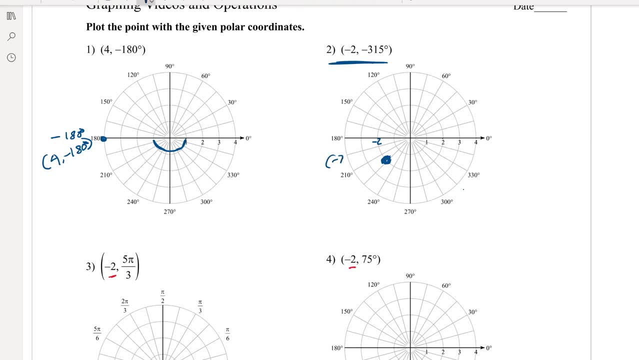 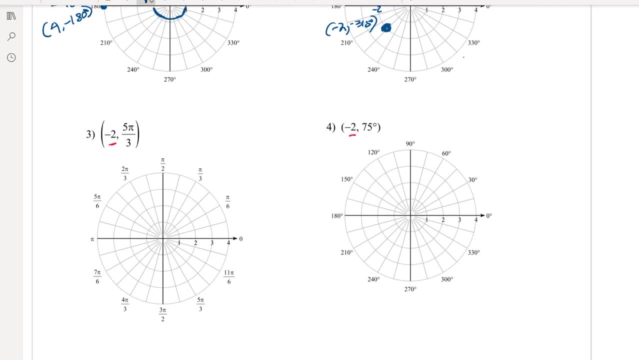 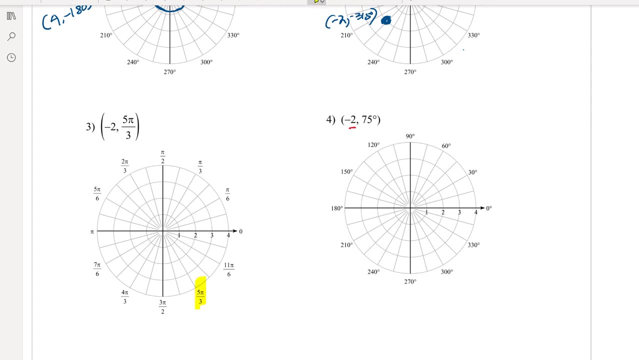 So the point radius negative 2, negative 315 degrees is right there. All right, Now you've got a negative radius but a positive. Well, 5, 5, 3rds is right here, And specifically 2, 5, 5, 3rds is right there. But the problem is we have a negative. so we're going to take this. 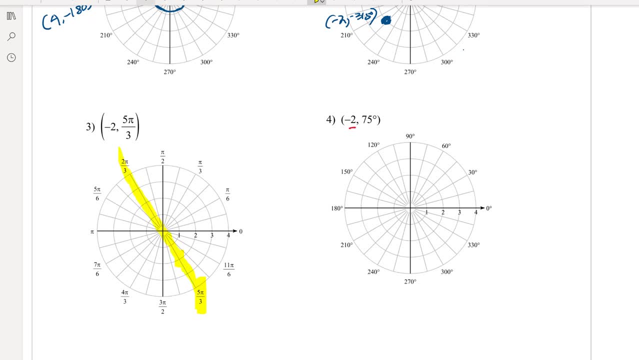 and we're going to follow it and I'm gonna, I'm going to locate negative 2, and I'm going to follow that around the circle until I get to 2 pi-thirds and that angle right there is negative 2, 5 pi-thirds. alright,